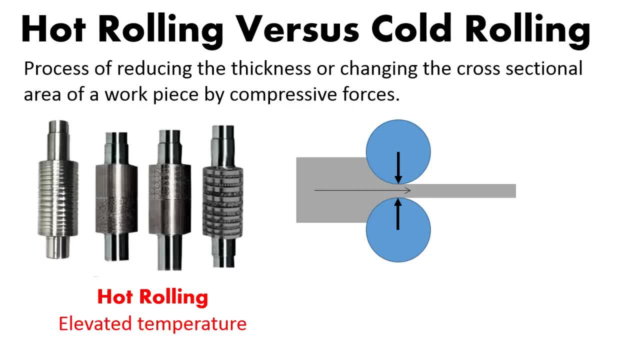 as the name implies, takes place at elevated temperatures. so we talked about this in another video and you can go check it out and see where i talked about forging. this takes place at above the recrystallization stage. cold rolling, on the other hand, takes place at room temperature. 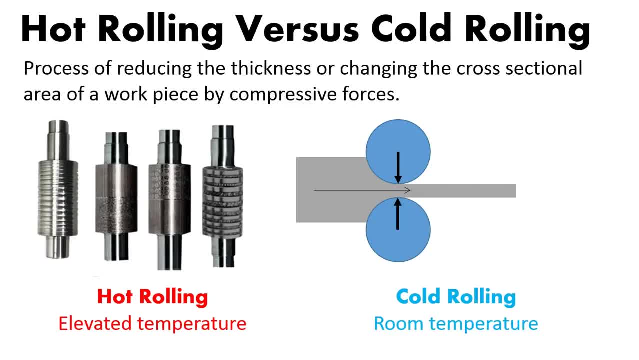 also along with cold rolling is it does have to go through a hot rolling process to get to this point before it goes through that cold rolling process. so there are more to cold rolling than just taking a piece of metal and rolling it out. so let's talk about both of those two processes. so 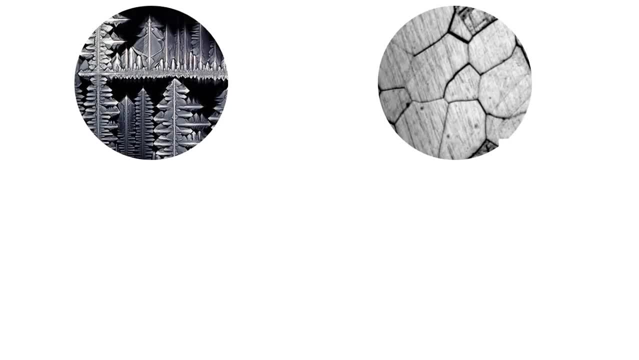 so for hot rolling you have a metal that goes through the recrystallization phase, so you heat the metal up and you end up on the left side here where you've got crystals. so these crystals have a name, they're called dendrites and as metal starts to cool and solidify, the crystals start. 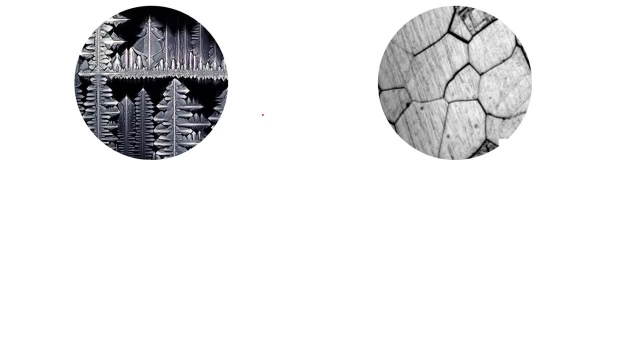 to reform and as metal starts to cool and solidify, the crystals start to reform and they form into grains. you see here on on the right, and when metal actually has been recrystallized it doesn't actually form into nice, neat little crystals. as you can see the crystals. 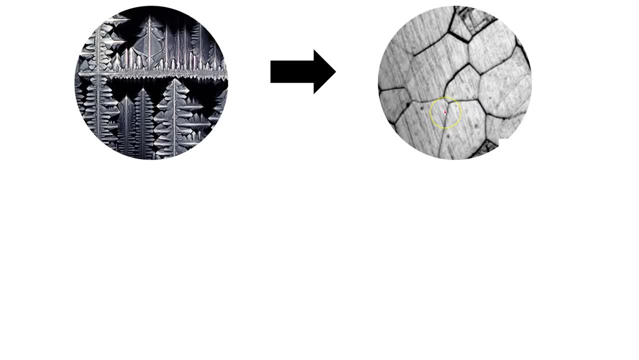 are in, uh, pretty much disarray. they're different sizes, there's gaps, there's- uh no, no real alignment, so they're real randomly oriented. so again, so you got these dendrites in these grains. so what they do is they heat the metal up above the recrystallization point. so 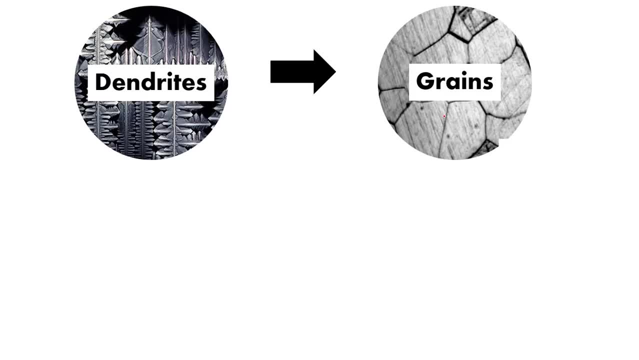 you actually are going back to dendrites, where you're actually going to be able to reform these into grains, and what you have is this whole hot rolling taking place at these elevated temperatures. so you're above recrystallization and what you do is you actually start to reform the grain. so 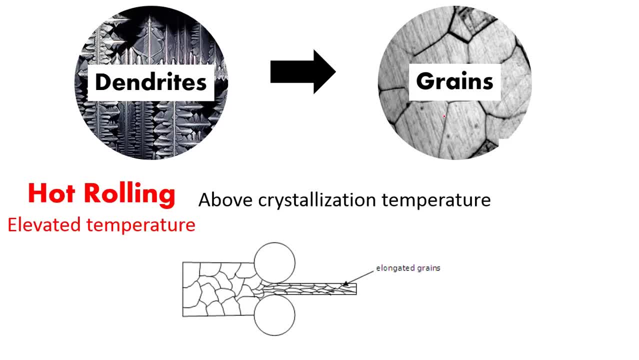 they're going through those rollers at the high compressive forces and you end up with smaller, more aligned grains, which makes the material stronger, much more harder and, much you know, change the metal property so that they are much more useful to you in your design efforts. so this is what the crystals start to look like. so 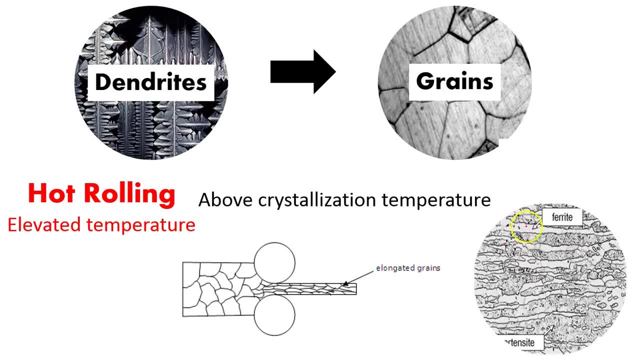 you can see, you've got a lot more alignment in your crystals than you do before the process. so here you have an after a hot rolling process, and up here is before the hot rolling process. so much more alignment on a much tougher material and much harder material, much stronger material. 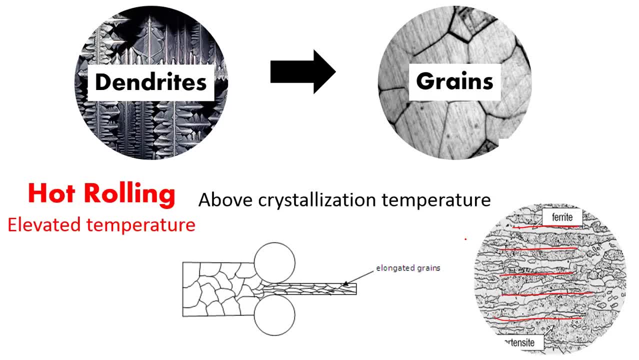 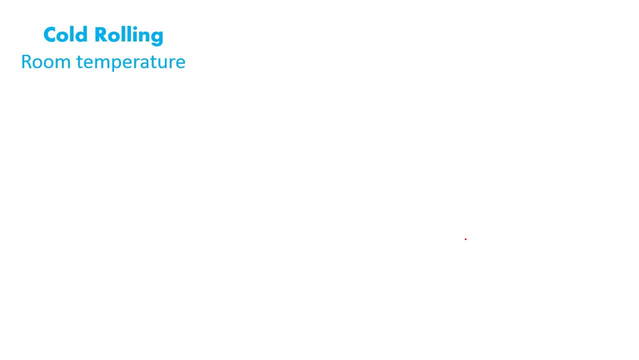 than an unrolled, unrefined grain. so what is cold rolling? cold rolling is done at room temperature, so you have a material that's actually been hot rolled, so its grains have already gone through some alignment process. now it's going through further processing, where it's actually getting rolled further with you. 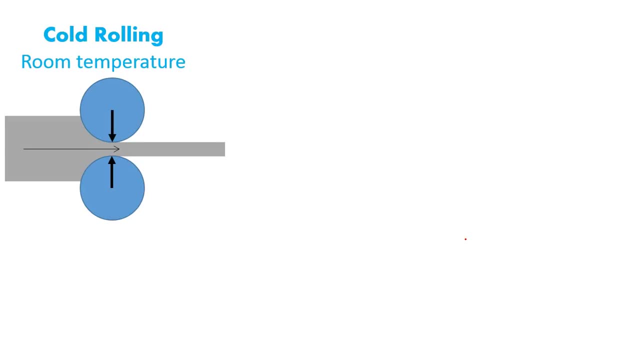 know high compressive forces. so we have the same rolling process that we looked at before. only now it's going through progressively rolling processes, so it's not just going through one, it actually needs to go through several because of the state that the material is in. so it's below the 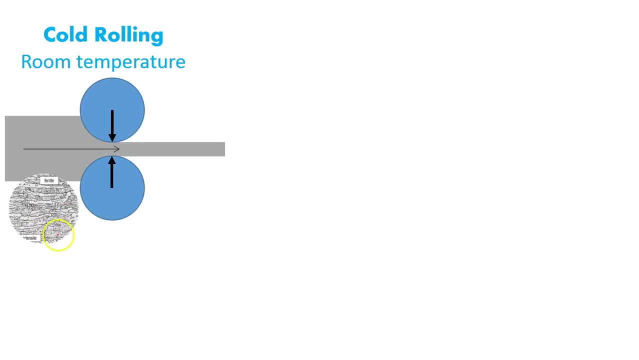 the request, the recrystallization phase. so here is the pre-formed, already rolled, hot rolled steel realigned grains going through this process and now something unique is happening. so since this has happened at room temperature, since the metal has already been formed once, we're going to look at something called a stress steering diagram now. i went through 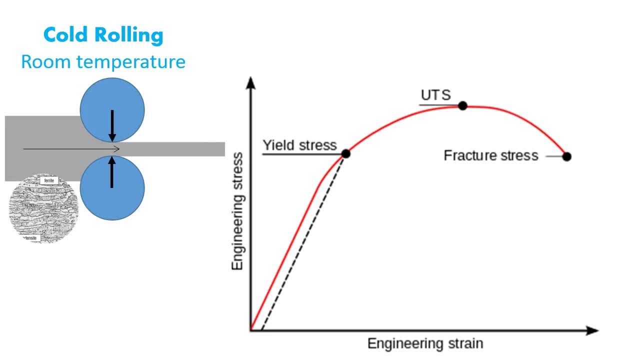 this in one of my strength and materials videos. i'll put up a card or a link for you to see that, but this is the stress during diagram. so on the x-axis we have the amount of strain and on the y axis the stress that you're putting the material through now as the material goes through this. 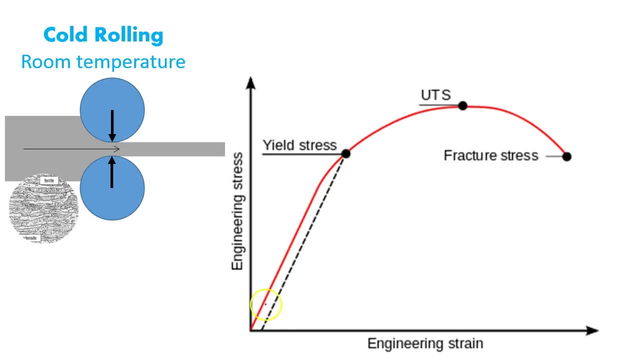 stage. this is called young's modulus or the proportional, you know the proportional limit on the material. this is where the material, as you start to put it under stress, it actually goes through a proportional amount of strain and it can always recover when it's in this stage. all right. 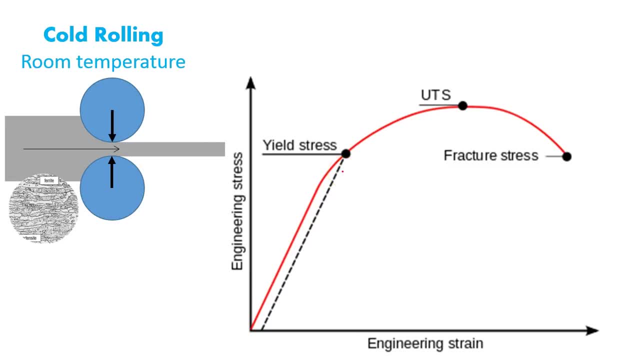 once it gets to this yield stress, something unique happens: it actually starts to get to a point where it starts to go back to its original shape. now, when it's in this state, it's known as strain hardening, and you can actually form the material or shape the material or stress. harden the material. 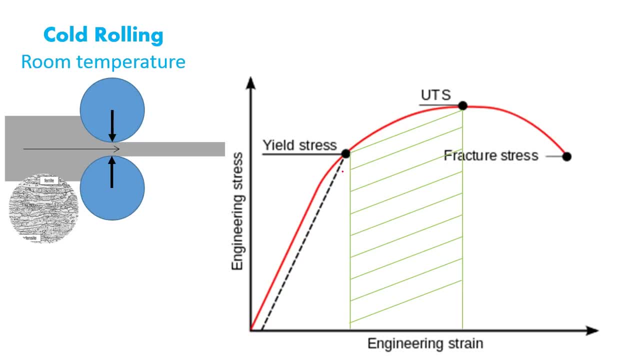 or work harden it. all these different terms and they all mean one thing: that the more stress you put under this material, the harder and the tougher it will become, and the material will keep getting harder until it reaches this ultimate strength, which is known as the ultimate tensile strength. 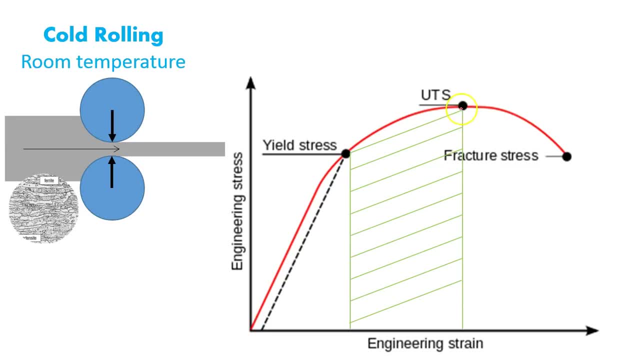 of the material at that point. it's a strong and as hard as the material ever is going to be. it'll never recover back to its original shape, but it is actually stronger and able to deal with a lot more stresses at this point. after this it's actually going to a phase called necking and it's prone to fracture. 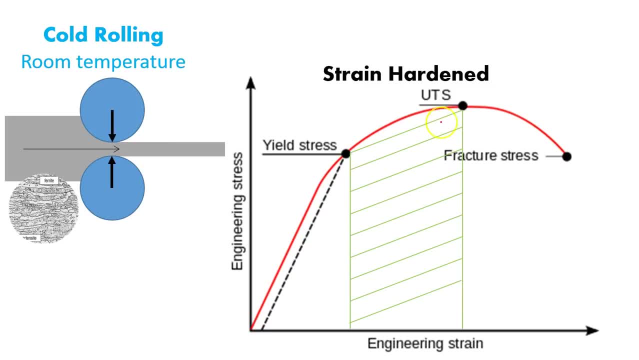 so in this stage, which is where cold rolling takes place. so this is the area we know as cold rolling. so that's cold rolling and that's where this is all taken place, right here in this green hatch mark portion. now, some of the benefits of it is it's actually, you know, stronger than hot rolling. it's more. 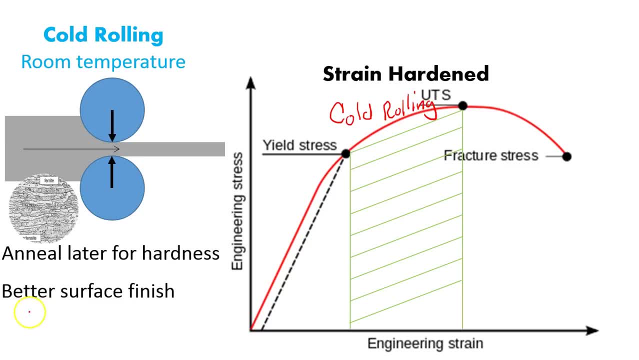 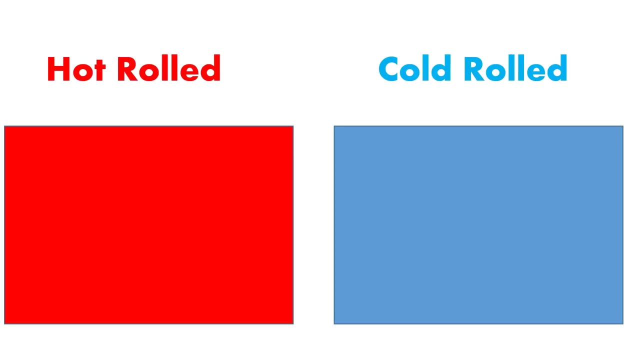 precision than hot rolling. it's actually got a better surface finish than hot rolling processes. it's also about twice as expensive and it does need to be annealed later to control the hardness and you also get much better precision. so those are some of the difference between hot rolling. 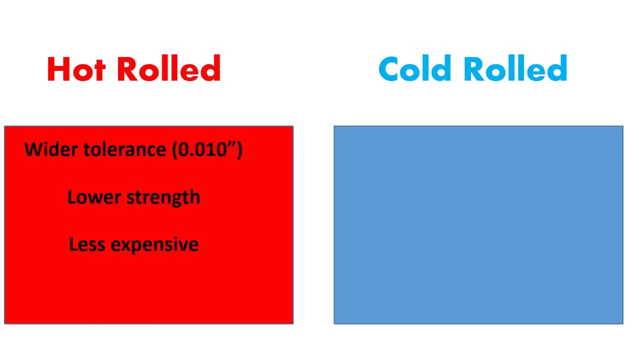 and cold rolling. so just to summarize things up. so hot rolling you have wider tolerances, so it's ten thousandths. it actually has a lower strength than cold rolling and it's less expensive than cold rolling. cold rolling on there has tighter tolerances, so about twice as tight. so five thousandths high strength and high hardness. 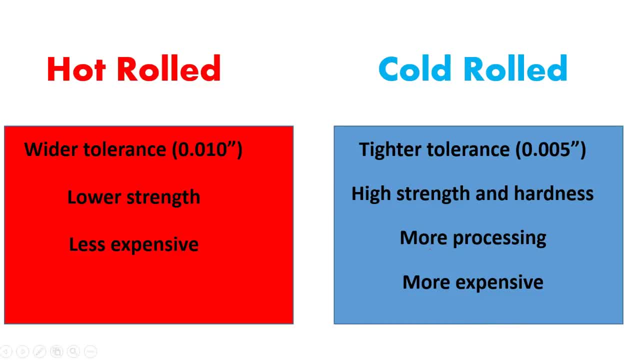 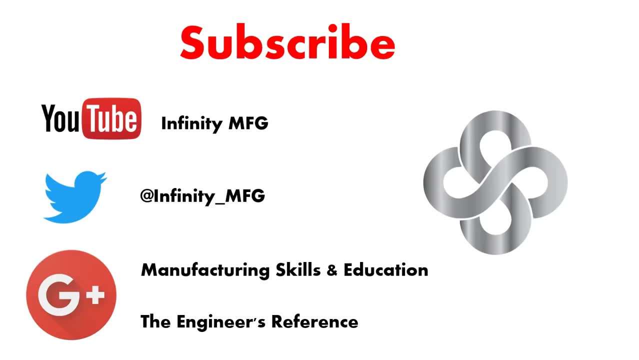 it does require more processing and it is a more expensive process. so if that video was helpful to you at all, go ahead and subscribe to my channel. i do videos on, as well as different engineering topics. please share the video to anyone you think might be able to benefit from it so you can subscribe to me on youtube. you can also follow me on twitter. 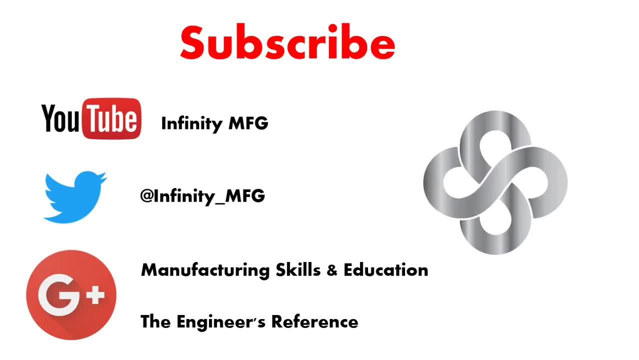 where i go through a lot of different uh, engineering and manufacturing topics up to date, talking about the skills gap and industry 4.0 or the fourth industrial revolution. you can also follow me on google plus. i have two fairly active communities. one is manufacturing skills and education, where i talk about, obviously, manufacturing and manufacturing skills.